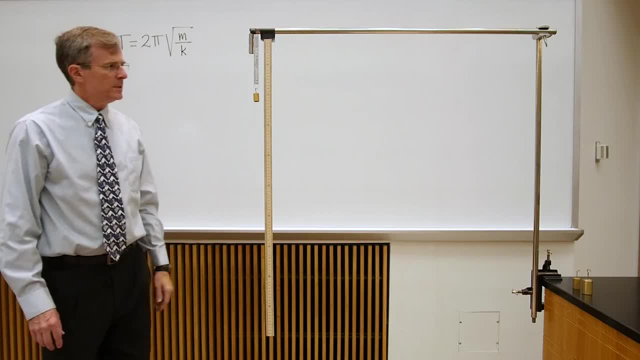 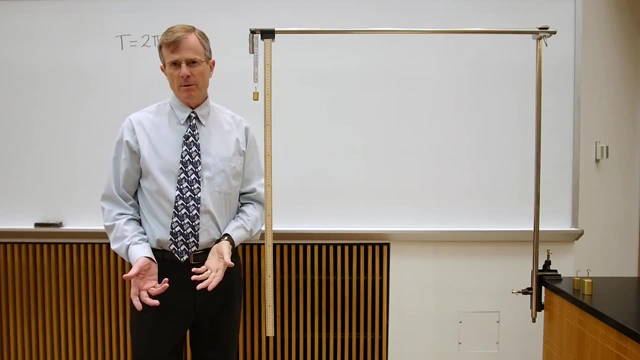 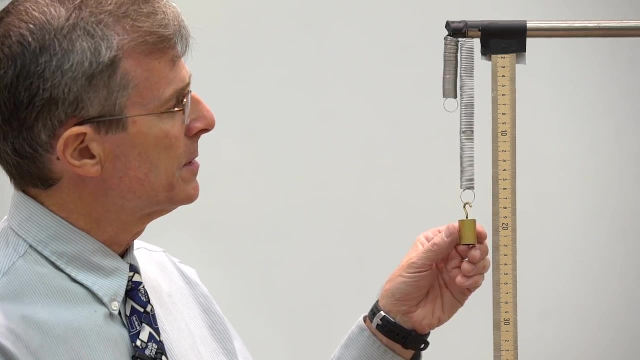 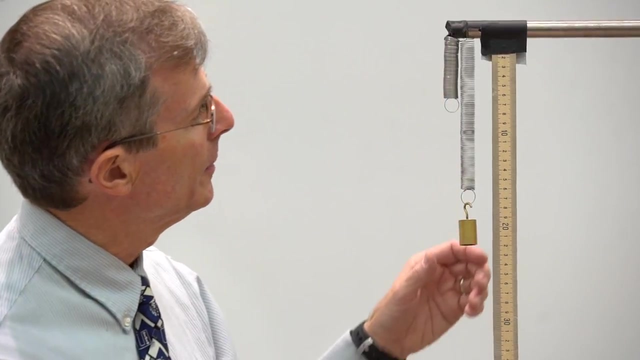 The other important parameter is the angle, The amplitude of the motion. In order to determine the amplitude, you have to first figure out where the equilibrium position is, And that's the position at which this mass is not moving at all. So it looks to be at about 19 centimeters from the support up here. 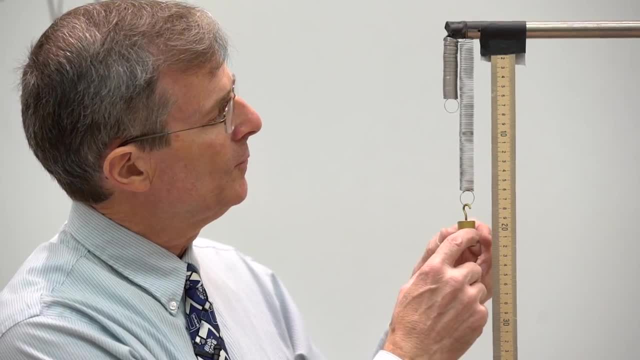 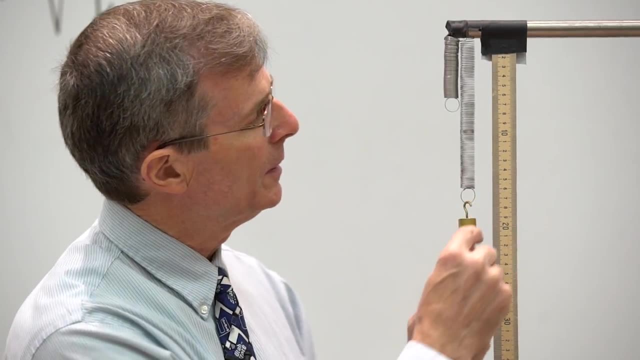 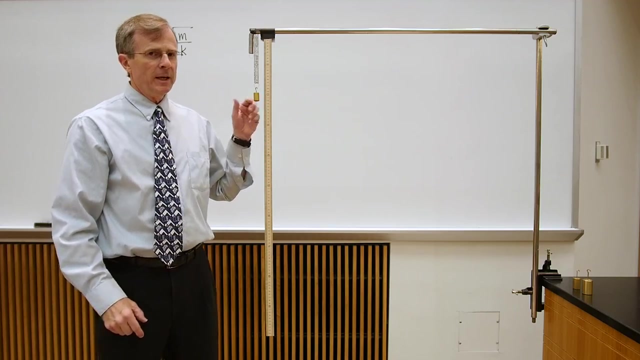 The amplitude is defined as the distance between the equilibrium position and I'm talking here about the top of the of the brass cylinder, here where it meets the meter stick here at about 19 centimeters. The amplitude is defined as the amount of excursion from the equilibrium position. 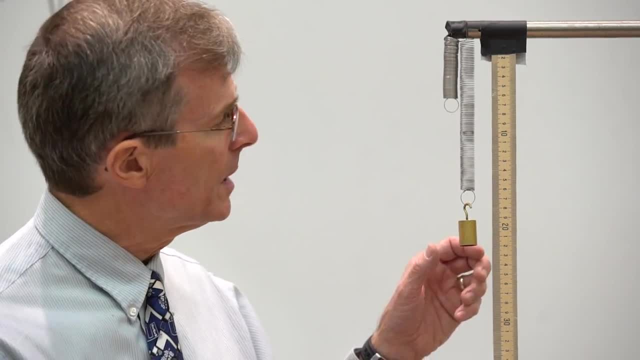 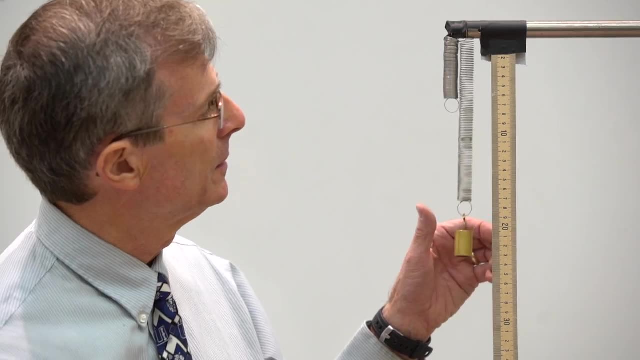 So to create an amplitude, a motion with an amplitude of 1 centimeter, I'm going to want to move this mass 1 centimeter up and release it, And so now it's oscillating roughly between 18 centimeters and 20 centimeters. 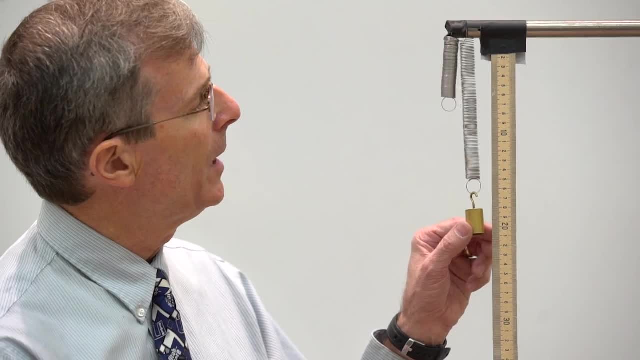 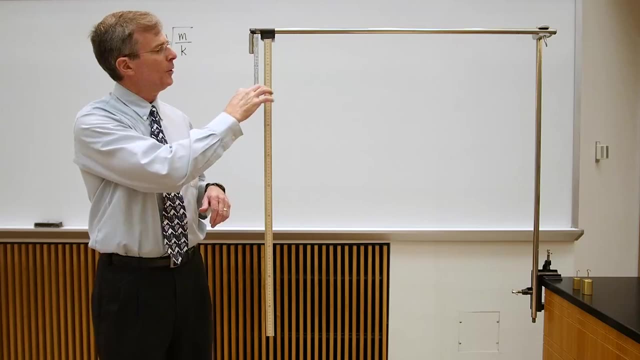 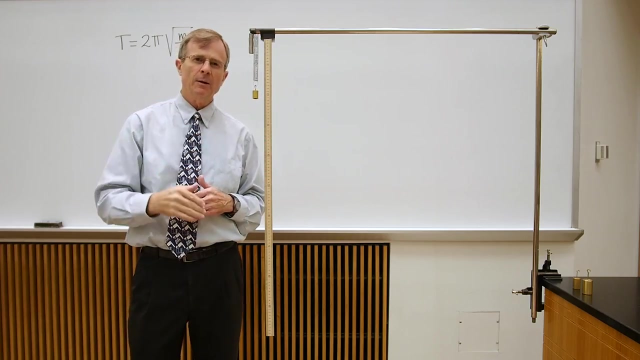 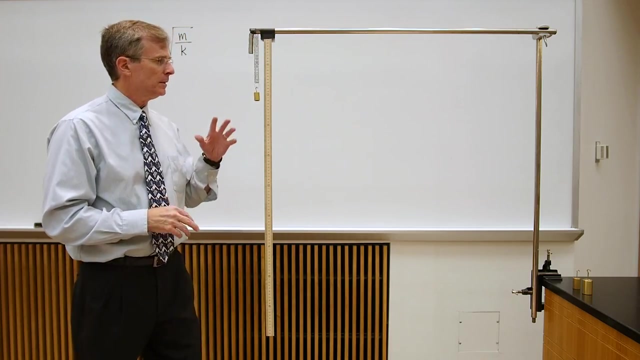 I could have done the same thing by moving it down to 20 centimeters, And then the overall motion is still 2 centimeters from top to bottom, but only 1 centimeter between the equilibrium position and one of the maximum positions. So now we want to look at the dependence of the period. 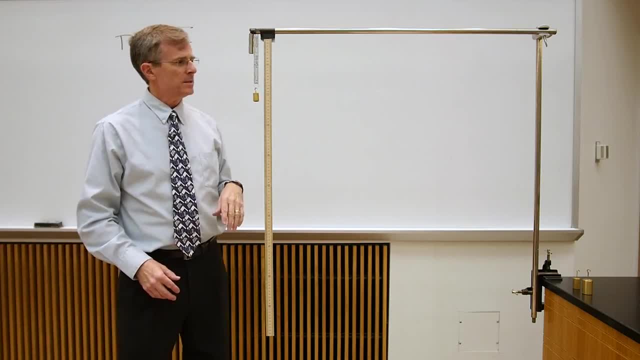 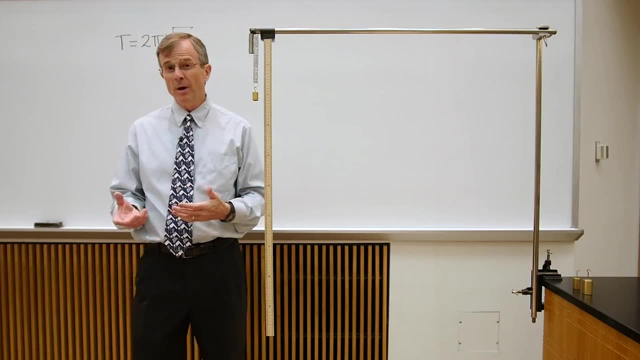 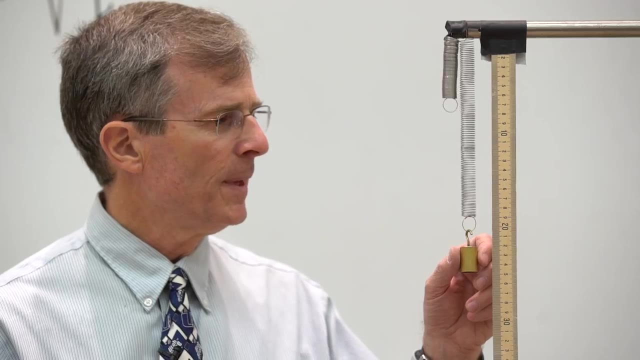 on the mass and the spring constant and also the amplitude. First the amplitude. And in order to just get a rough idea about how the period depends on amplitude, then let me look at a couple of different amplitudes. Here's a fairly small amplitude. 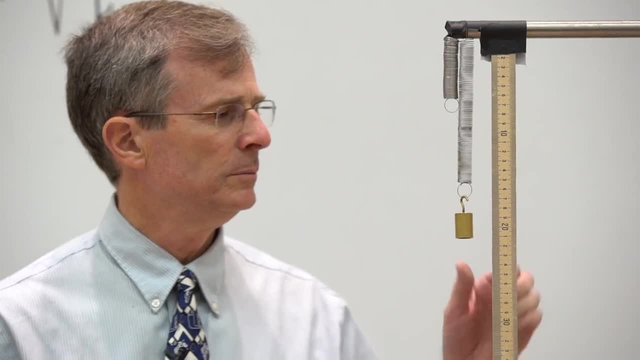 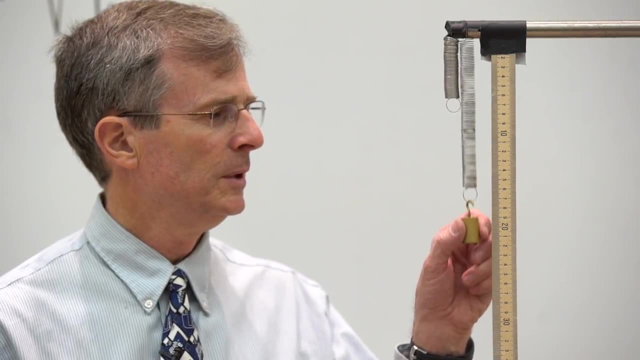 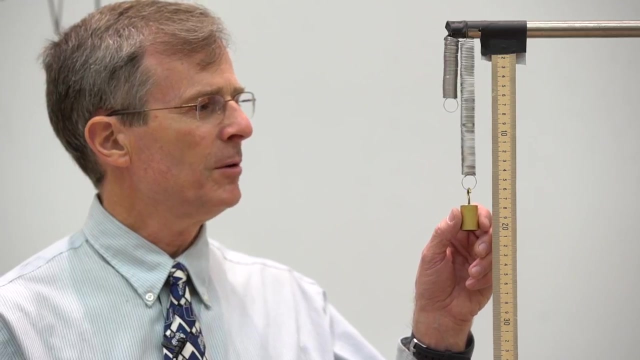 Boom, boom, boom, boom, boom, boom. Here's a medium amplitude: Boom, boom, boom, boom boom. And here's a large one: Boom, boom, boom, boom, boom. And back to the small one again. 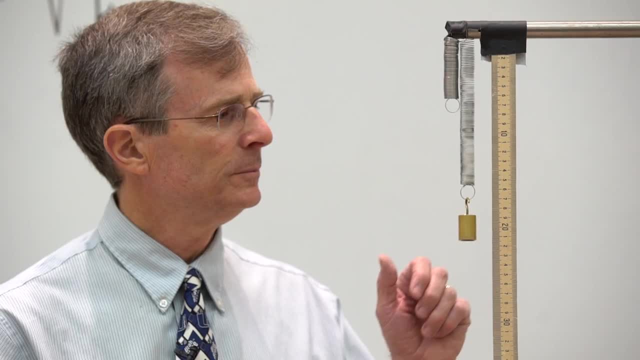 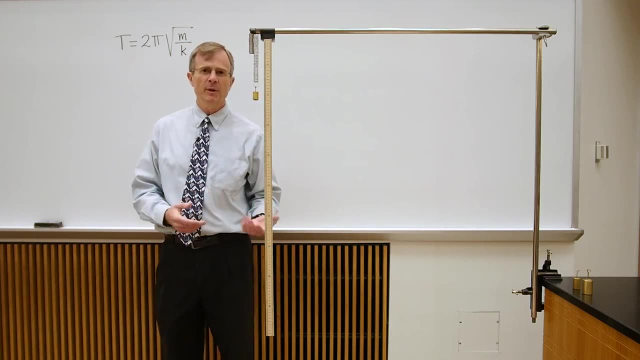 And we're just getting a rough measurement here. Boom, boom, boom. I think you can tell that the amplitude, or that the period doesn't seem to be depending much, if at all, on the amplitude, And in fact the mathematics bears this out. 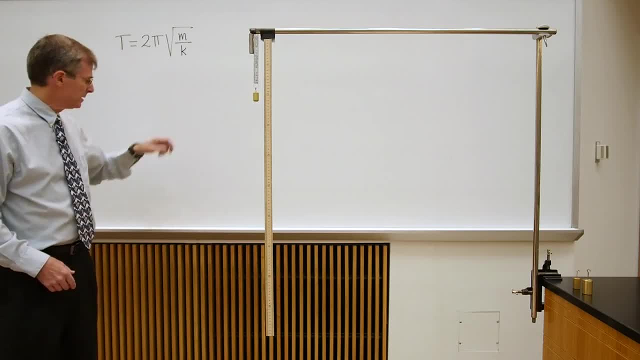 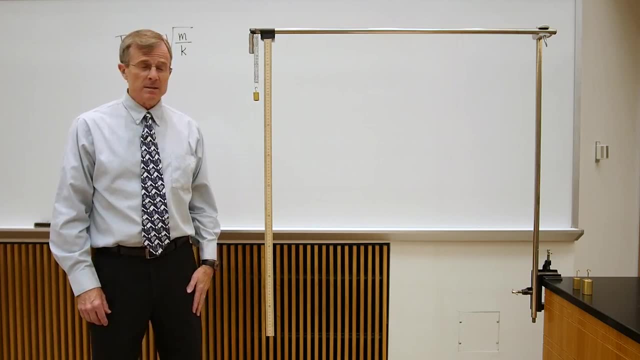 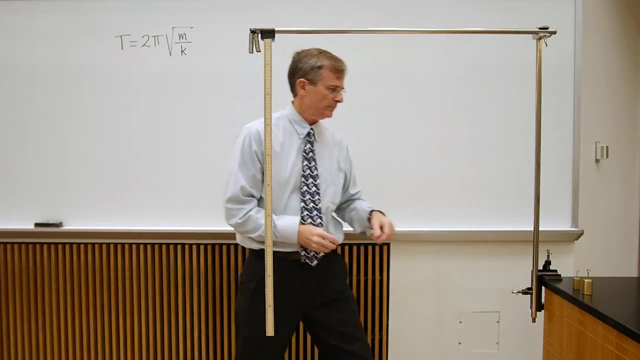 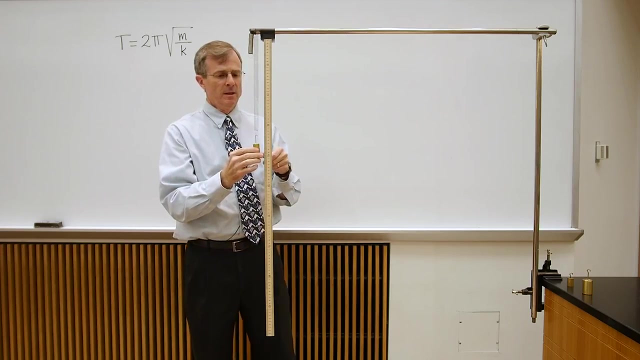 The period t has no dependence on the amplitude of the motion, But it does depend on the mass. So let's look at the period as a function of the mass. by adding a bigger mass, You can remember how fast the last one was going. 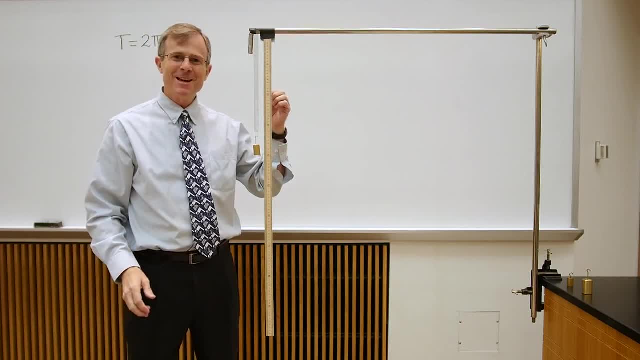 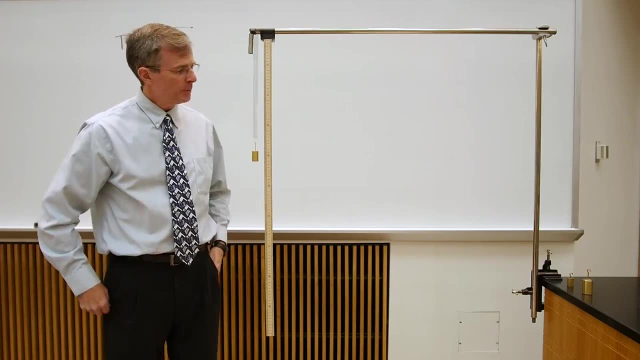 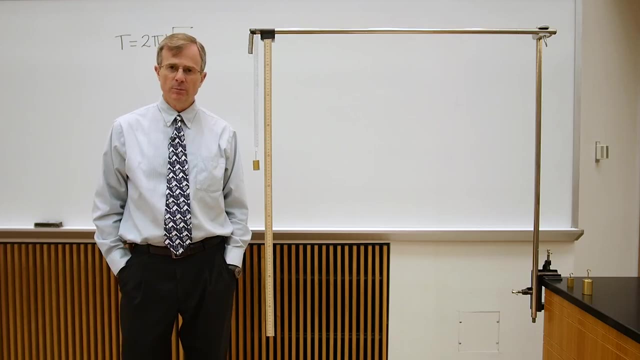 First thing to notice is that our equilibrium position is no longer at 19 centimeters, It's down at around 36 centimeters. And then, if I give it some motion and look at the period, the period is now boom, boom, boom, boom, boom. 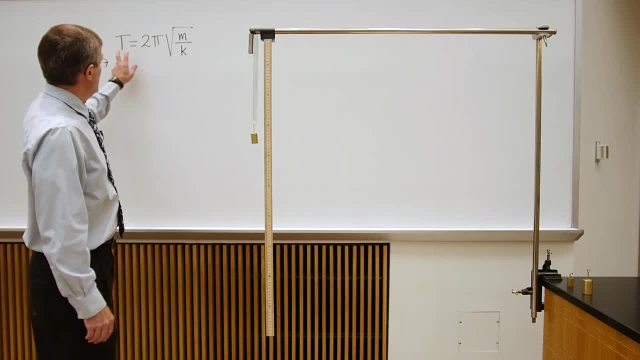 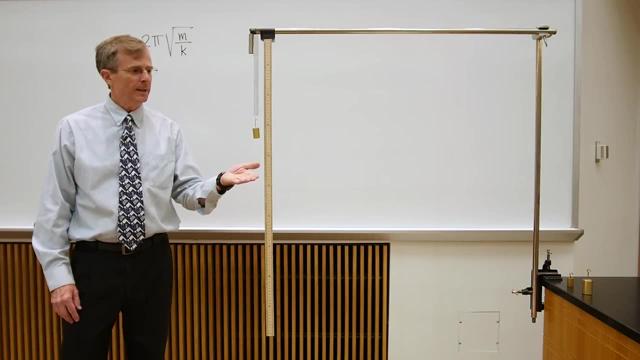 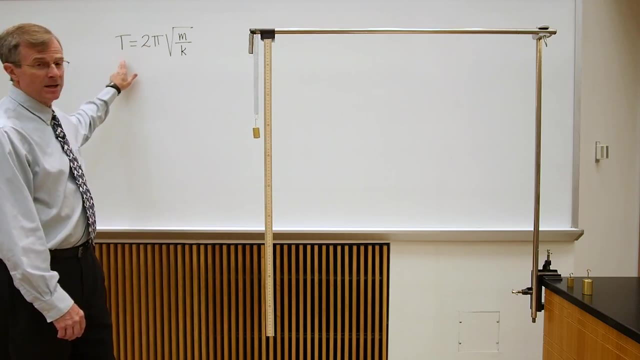 It's slower, It takes longer. So that means the period is the time between a time for one complete oscillation. So that's from here Back down to here again. That time is now longer with a bigger mass, Exactly as predicted by the equation. 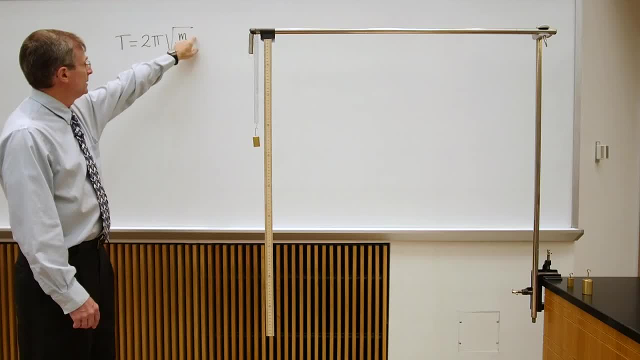 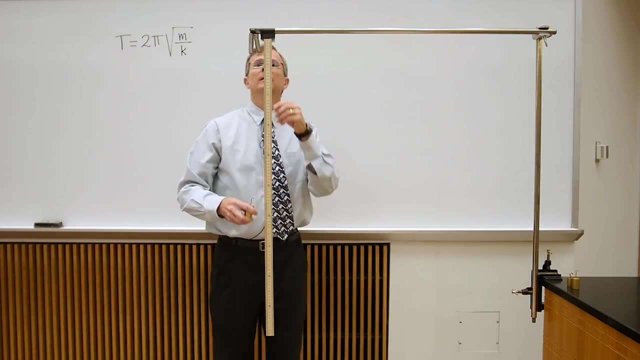 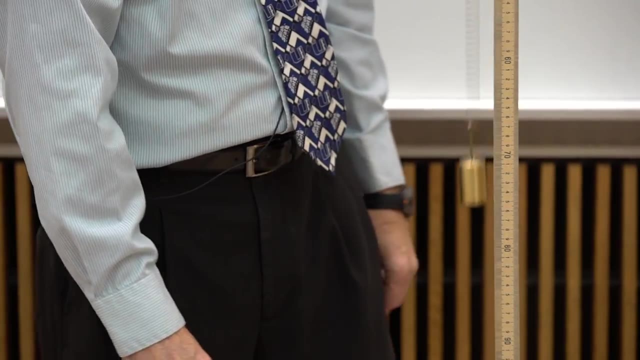 if you increase the mass, it's in the numerator here that will increase the period or the time for one complete oscillation, And then, bringing this to the extreme, even longer period equilibrium position: much lower. Boom, boom, boom. 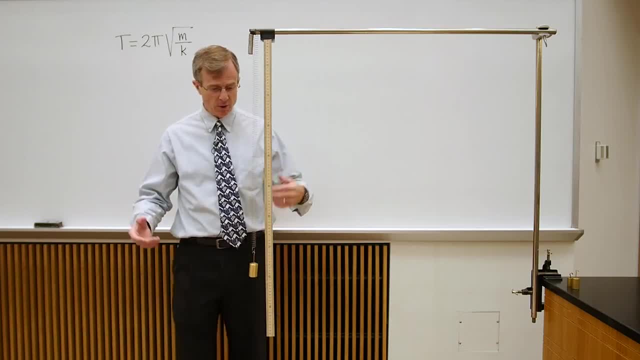 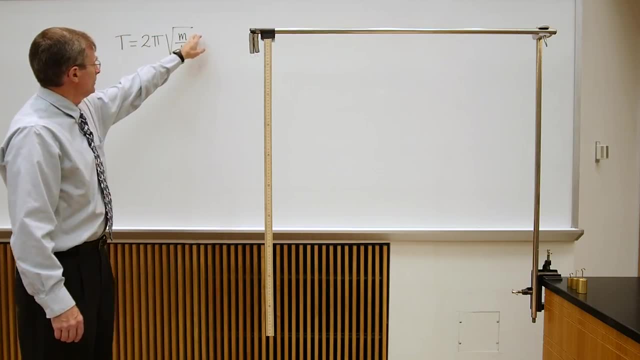 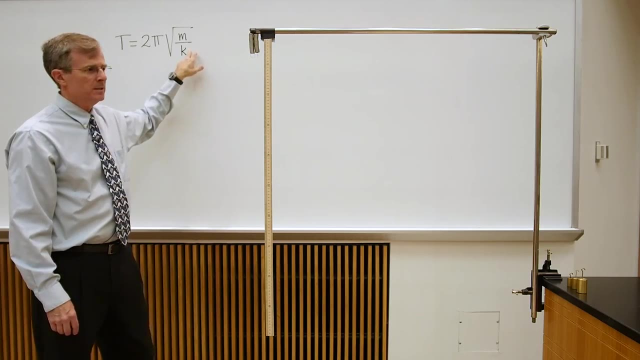 Boom, boom, boom. Very, very long period motion. So how does this depend on the spring constant? k Dependence on the mass down The period depends on one over the square root of the spring constant. If I use two springs instead of one, I thereby doubled the spring constant. 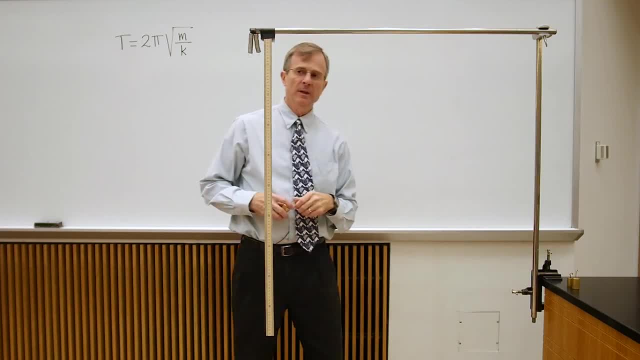 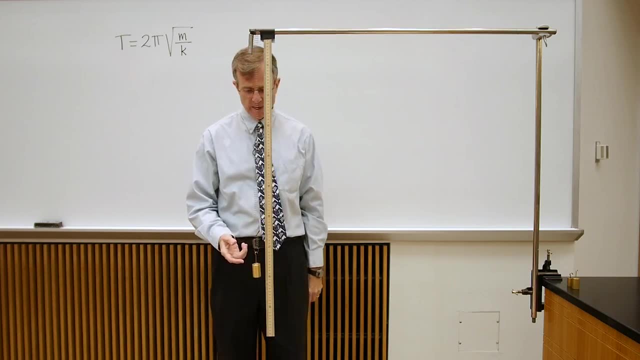 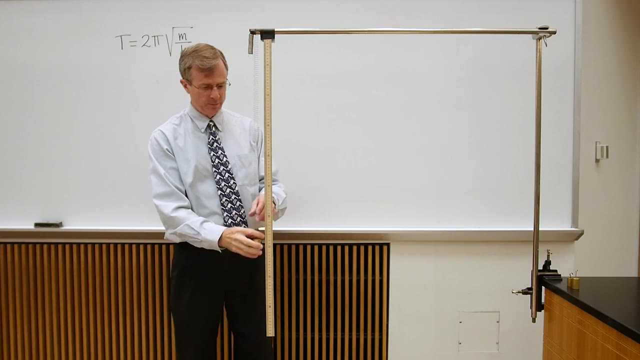 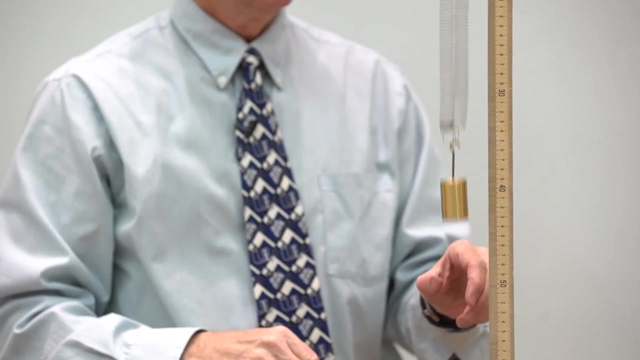 So let's compare the period With just one spring and this large mass- boom, boom, boom, boom- And the same mass with two springs. You know, first, that the equilibrium position is higher because we've got more force pulling it up to counteract gravity.